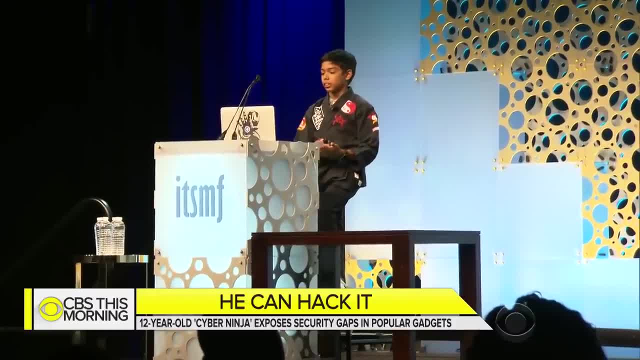 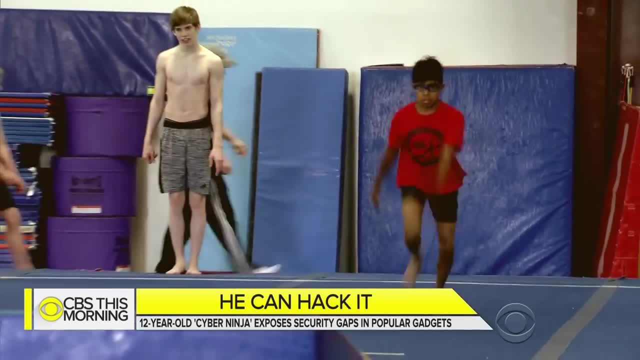 cybersecurity, because obviously what we have invented so far is clearly not working. This cyber ninja, as he calls himself, has a second degree black belt in kung fu and he's on a mission to show how hacking is child's play. If a 12-year-old can do it, what makes it that somebody? 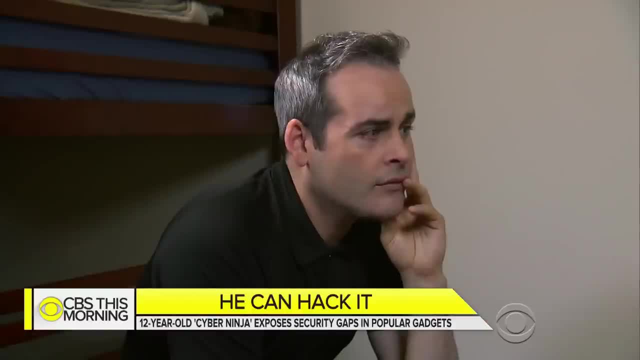 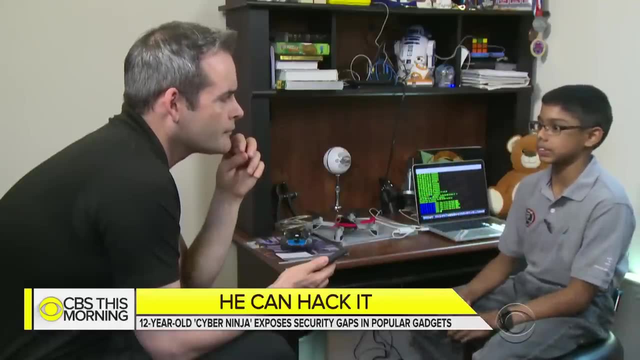 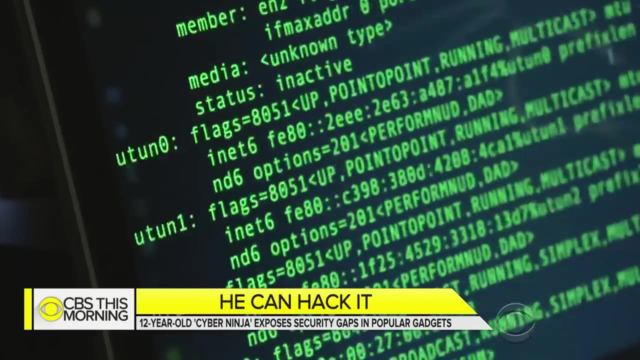 is a skilled, actual cyber terrorist. What makes it that they can't do it? This Bluetooth is going into new autonomous cars, autonomous drones. It's going into medical devices. Paul says that the Bluetooth and Wi-Fi connections that we use almost every day are extremely vulnerable to hacking. 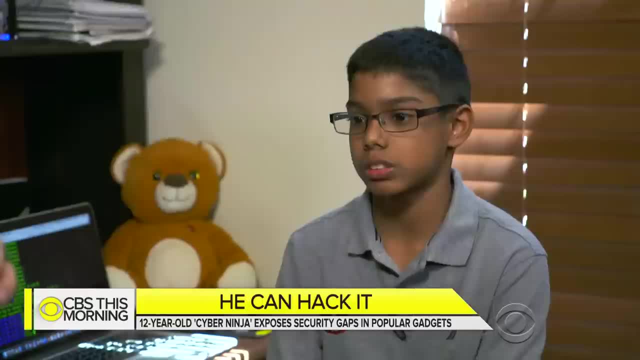 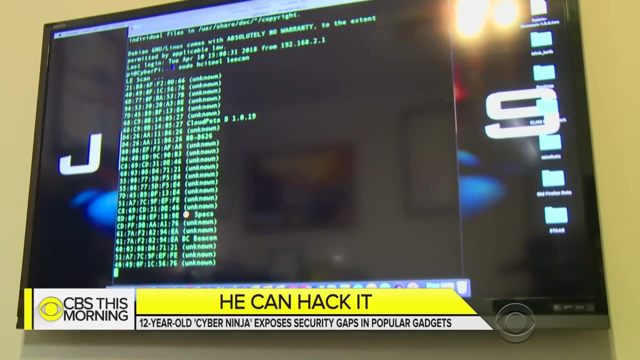 I'll never connect to a public Wi-Fi that I don't know. Really. Somebody can just hack into that Wi-Fi network and poison it. He showed me firsthand how a hacker's poison can spread from a Wi-Fi signal. I successfully know your password. How do you know my password? And I've hacked you. 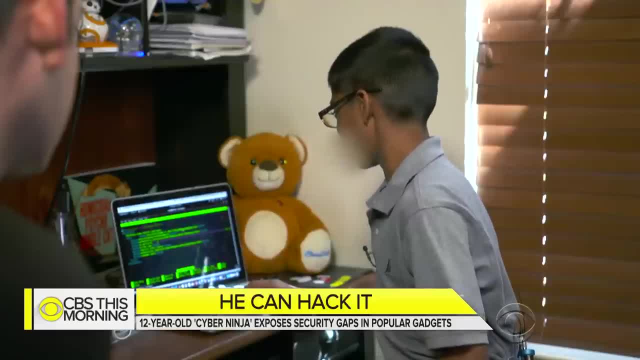 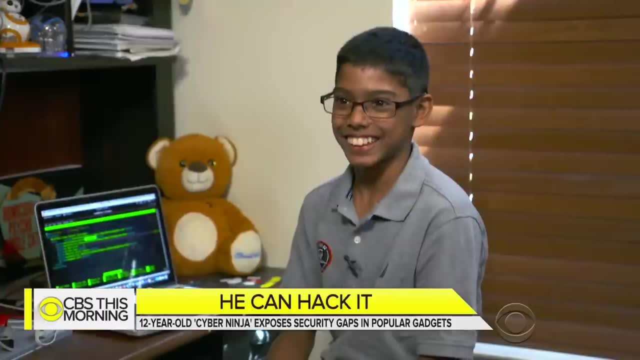 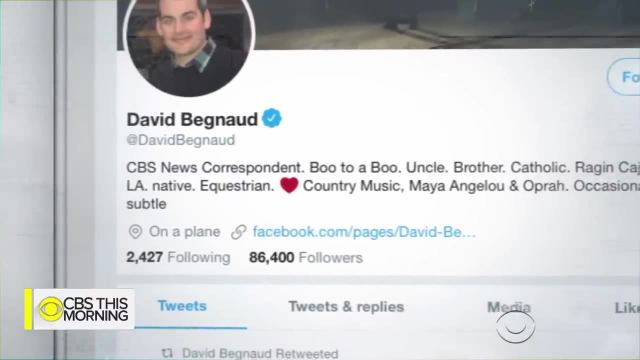 Your login was david. Yes, yes, yes, yes, yes, Yep, let's bleep that, Let's bleep that out. Wow, So, uh, call me gullible, You got me. It took seconds. He had my Twitter username and password using a fake page that he'd cloned. 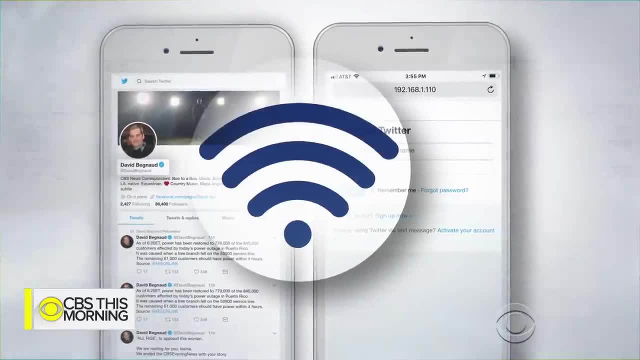 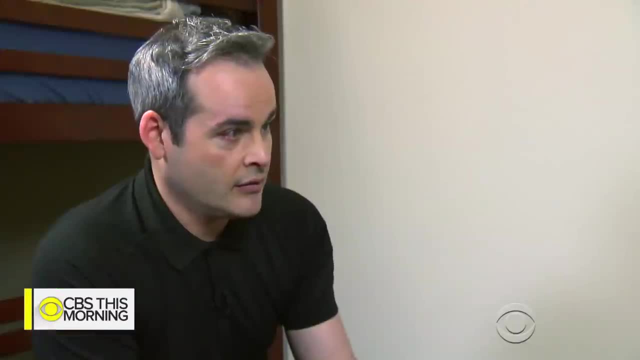 after I connected to his public Wi-Fi network. It's that easy. So, in other words, if I was sitting at a Starbucks, I went to sign into Twitter. I put it in. they got it. Now staying in touch is easy and fun. 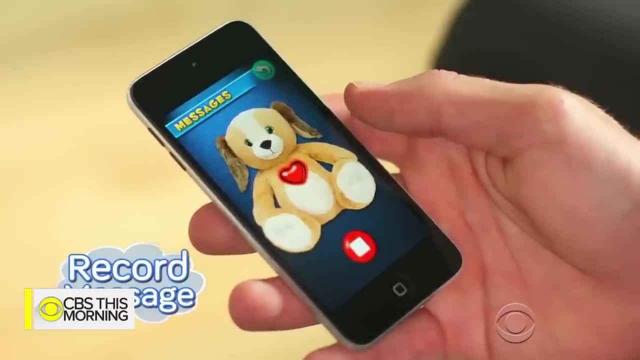 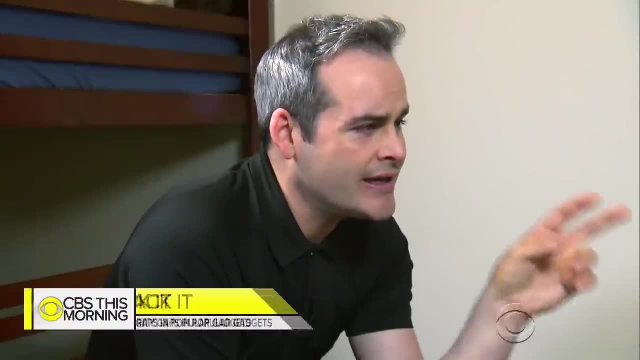 Paul also hacked Cloud Pet. It's Teddy Bear. It uses Bluetooth technology, allowing traveling parents to send messages back to their kids. What did you do that turns that into a threat Without any notification or any knowledge of the user? I could turn it on from my computer. 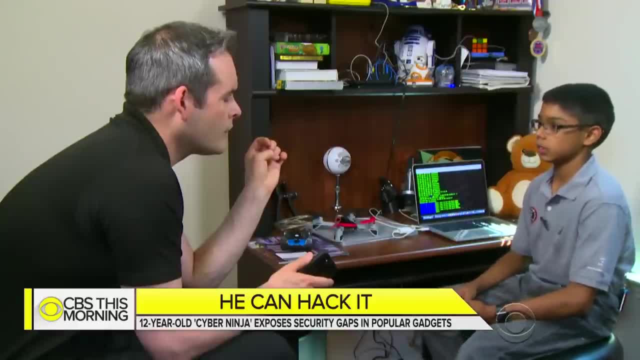 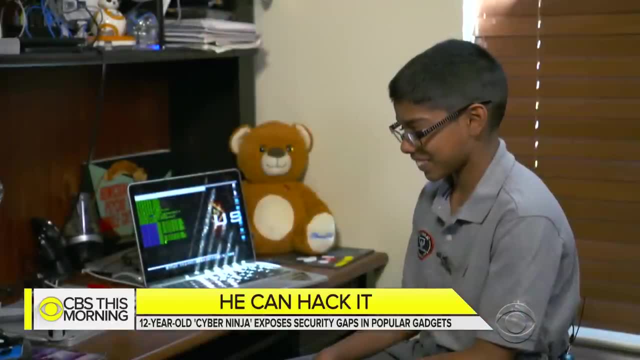 which only has to be in a 30-foot radius of the bear, So I could stand outside somebody's house. He turned the bear into a secret recording device. How do you get this thing? cyber ninja? Who's the smartest one in the family? 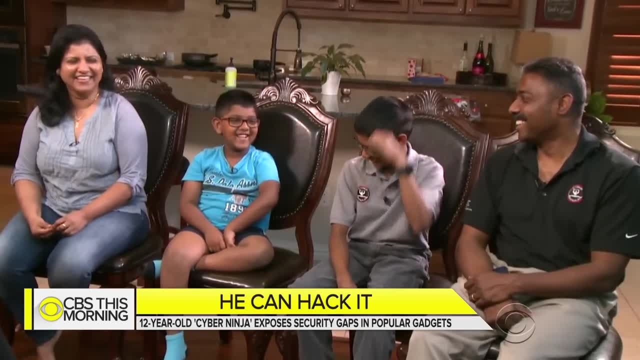 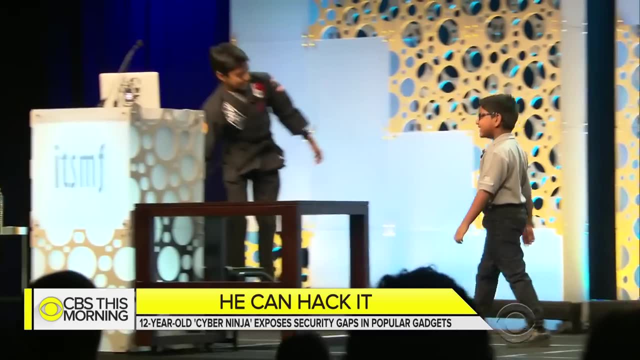 The Paul family of four is hopeful about the future of cyber security. Ruben's parents, Mano and Sangeeta, both work in technology, And his six-year-old brother, Itai, is even joining him on stage now. Can you show us this?